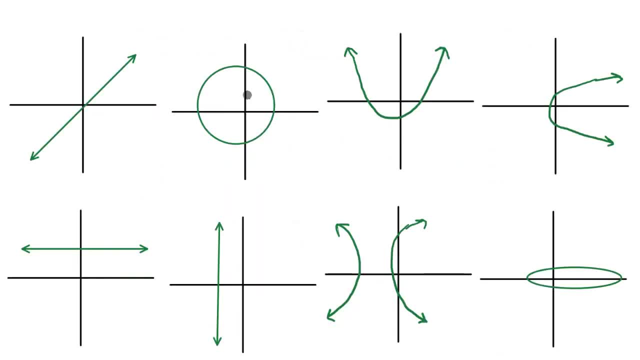 Here we have eight different graphs and we want to determine which one of these are functions and which one are not functions, And what we're going to do is use the vertical line test. and the reason why the vertical line test works is because every x value can only have one specific y value. 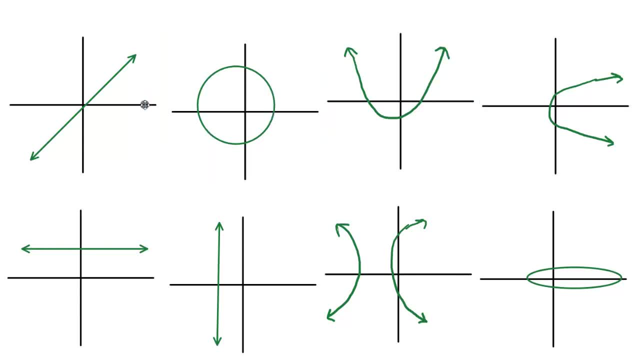 Let's go ahead and bring in this vertical line. So when I place this vertical line over this diagonal green line right here in this graph, it can only cross it one time. So as you see, as I move it from my right to my left, it's only crossing it one time And that means it is a function. So this first one is going to be a function. 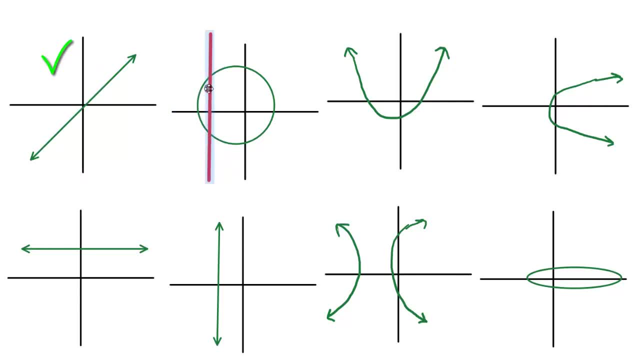 The second one: if we move it over this circle, you'll notice that the vertical line is always crossing it two times, So that means it's not a function, The only times that it would cross it. one point would be if you put it at the very end, like right there. 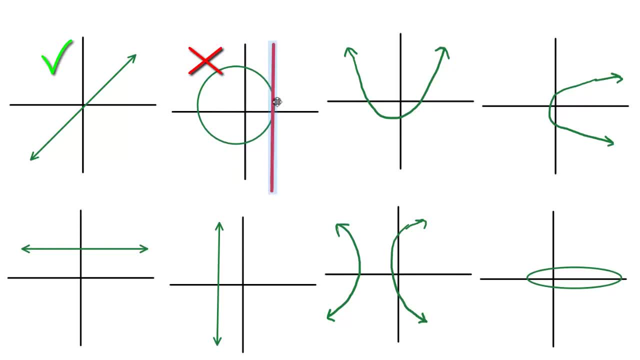 And if this vertical line was tangent to the circle, it would only cross it once. But still it's not going to be a function, because if you move it a little bit to the left then you'll see that it crosses it two points. 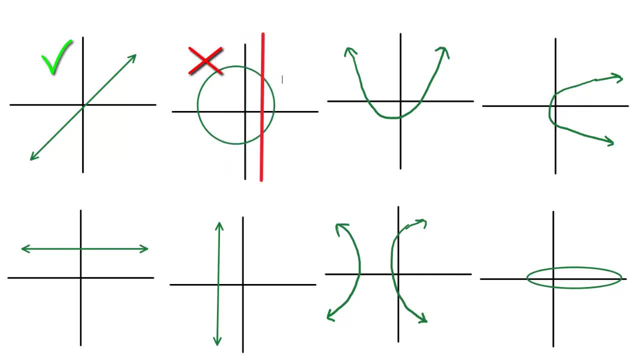 So a little bit more about that is, say, if I'm going to keep it there and I call out a point And I'm just making this up, But say this is one and then two, This point right here would be two comma. I don't know I'm making, say three, 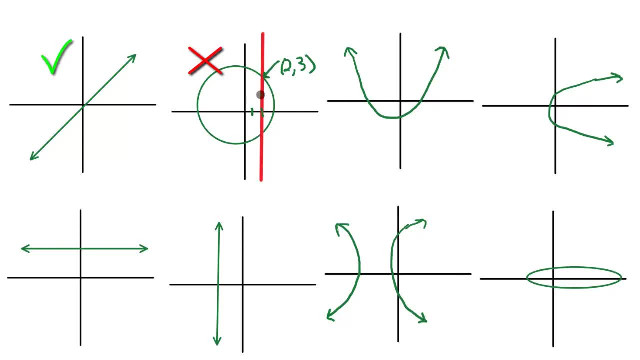 Well then this point down here has to have the same x value, right? We go over two times, So that's going to be two comma. I don't know. it would be negative, say, like negative three, And then if we plug two into a function, supposedly we'd get three, and then we'd get a negative three. 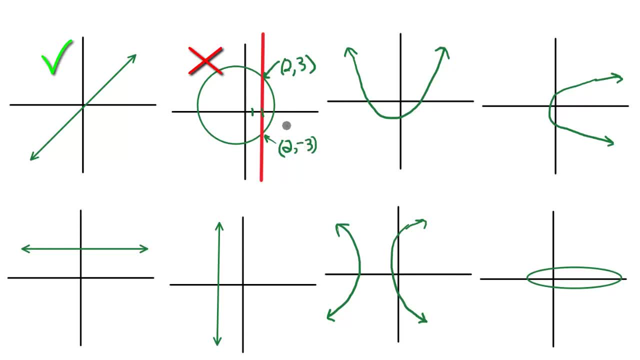 But that can't happen. You can only get one. So that's why it's a function, That's why it's not going to be a function. So let's go ahead and get rid of all this And we will move on over here to the parabola. 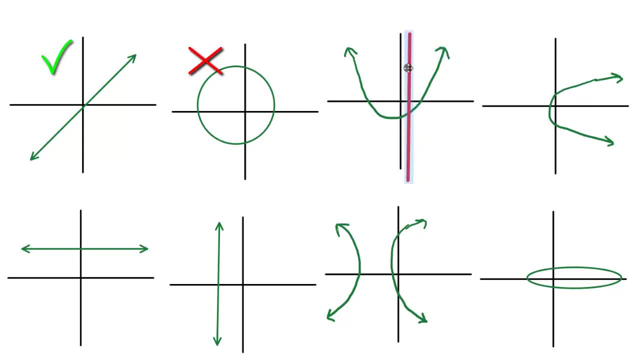 So I'm going to move this vertical line from right to left And you'll notice that it only crosses that one point. So this was a. this will be a function as well. If I move to the right for the sideways parabola, you'll notice that it's always crossing it two times.